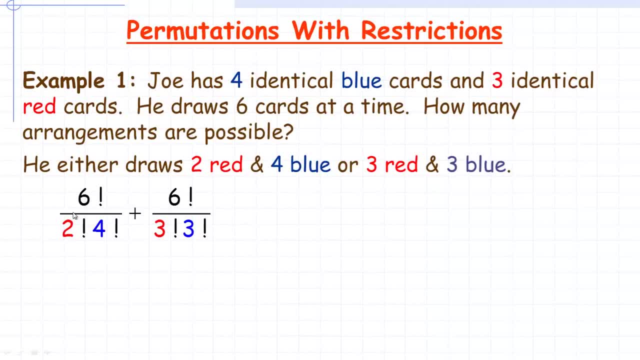 So, and there are of course all the blue ones identical, all the red ones identical, So we would take, excuse me, six factorials, Because there's six objects, and divide by two factorial and also by four factorial. 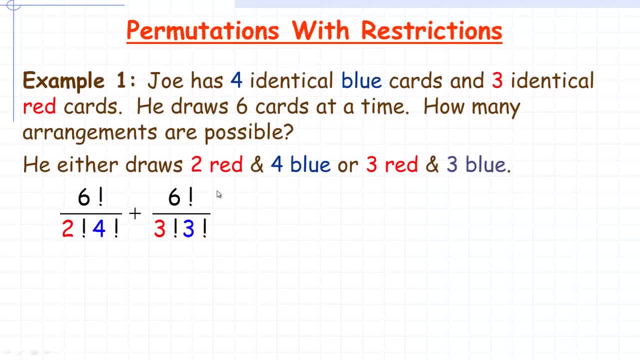 because these red ones are identical and so are those blue ones. And then, so that's the ways he can select: two red and four blue, And this is the calculation for how many ways he can select or arrange three identical red things and three identical blue things. 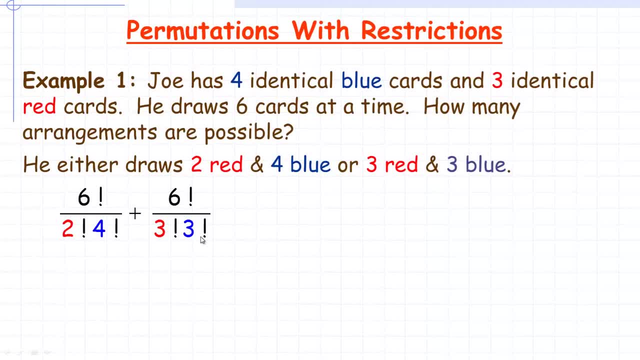 So we would divide six factorial by three factorial times three factorial And if you evaluate that, divide that out, this first calculation will work out to fifteen. So there's only fifteen ways he can select two red and four blue in different orders, And there's twenty ways he can select three red and three blues. 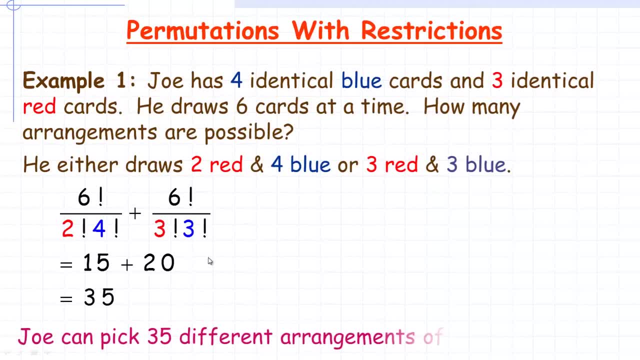 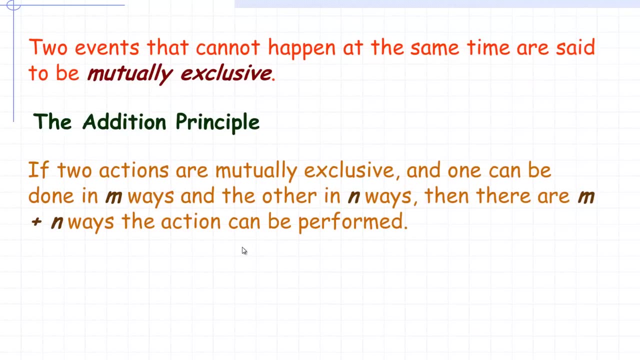 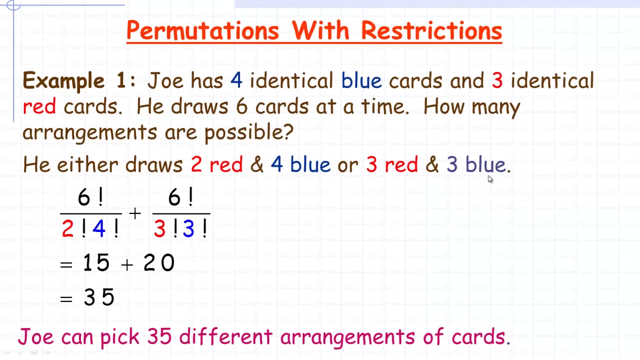 And of course that adds to thirty-five. So altogether Joe can pick thirty-five different arrangements of cards that are either two red and four blue or three red and three blue. Now two events that cannot happen at the same time. for example, you cannot at the same time select two red and four blue and also three red and three blue. 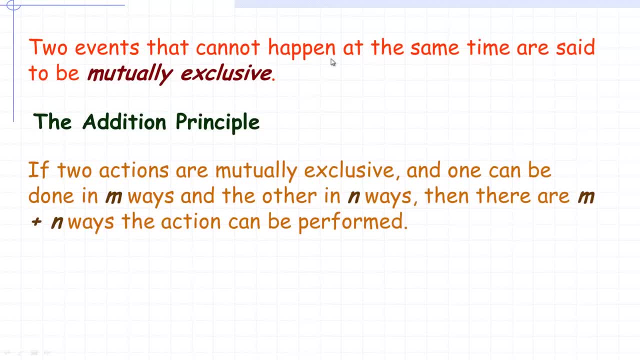 It's impossible to do that. Two events that cannot happen at the same time are said to be mutually exclusive, And so we get what's called the addition principle, If you have, if two actions- and this extends past two- are mutually exclusive, and one can be done in m ways and the other one in n ways. 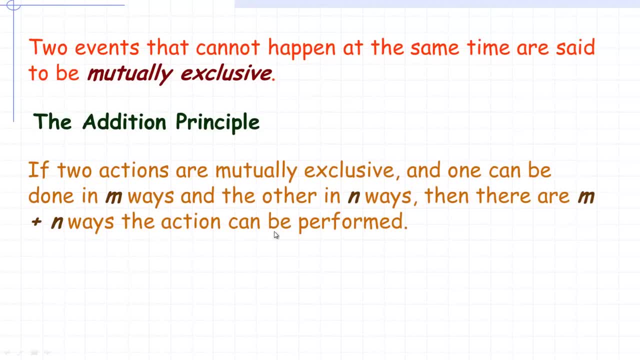 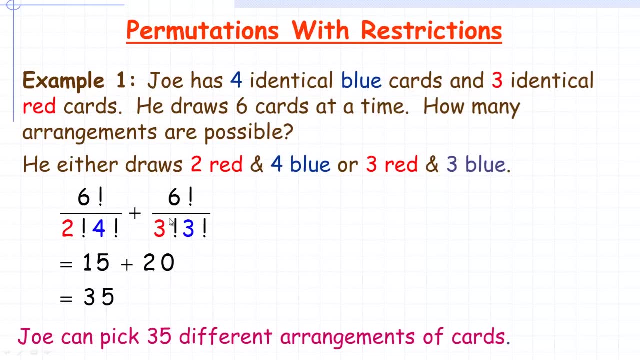 then there are m, M plus N ways the action can be performed. So that's why in this page we added the calculation for how many ways you can get 2 red and 4 blue to how many ways you can get 3 red and 3 blue, because they're mutually exclusive. 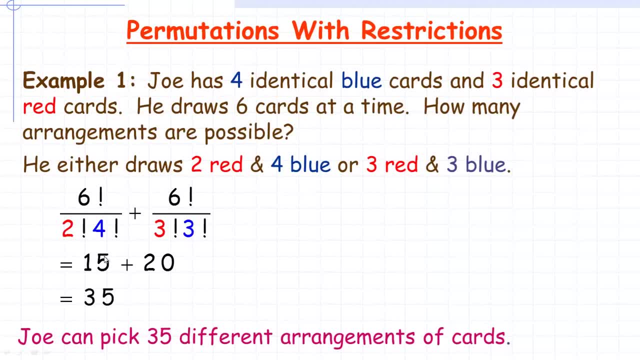 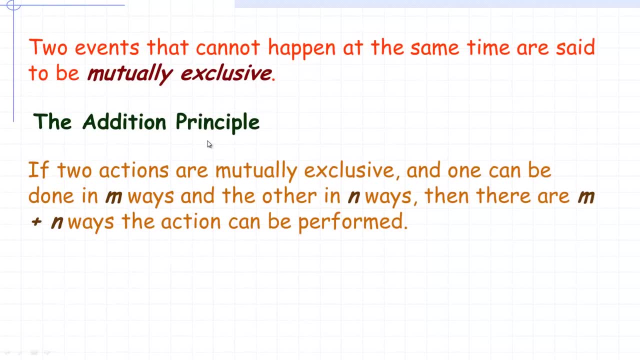 So that's why we added the 15 and 20.. There's 15 ways you can do it this way and there's 20 ways you can do it this way. so all together there's 35 different arrangements. So that's the addition principle for mutually exclusive actions. 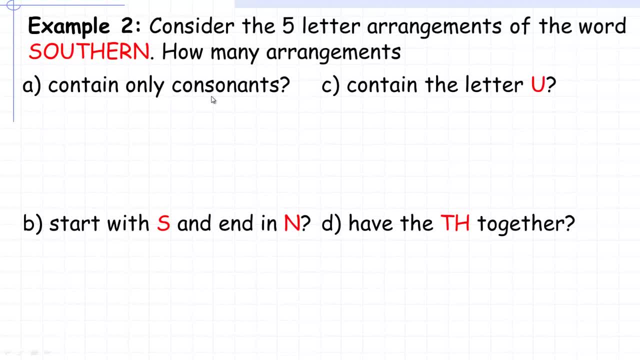 In example number 2, it says: consider the 5 letter arrangements of the word southern. How many arrangements contain only constants? So there's a restriction. Constants do not include, of course, O, U or E. So we're only talking about the S, the T and the H, the R and the N. 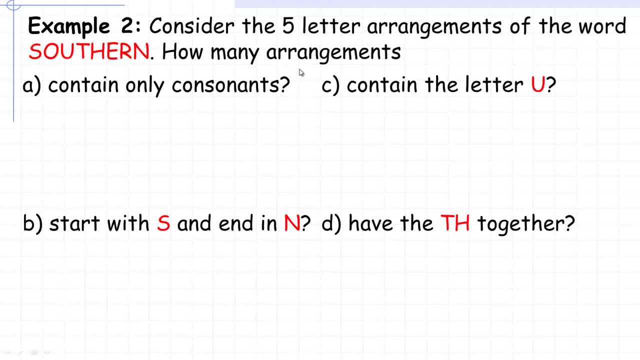 And here's another restriction too: We're only talking about 5 letters at a time, So there are 5 consonants. So well, I guess in that case we're actually arranging all of the consonants. So if there's 5 of them, we could arrange them in 5 factorial ways or 5 permute 5 would be the same calculation. 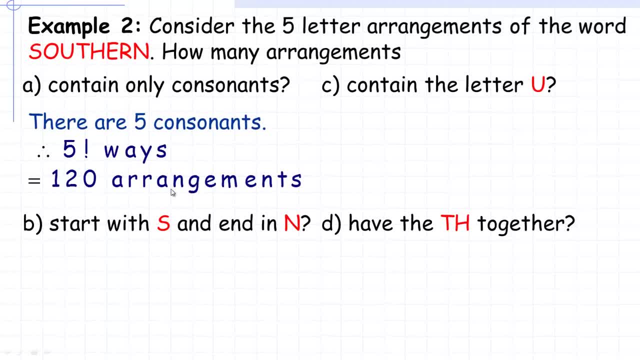 And 5, factorial is 120, so there's 120 different arrangements that contain only consonants. In B, it says how many start with an S And B says how many start with an S And B says how many start with an S. 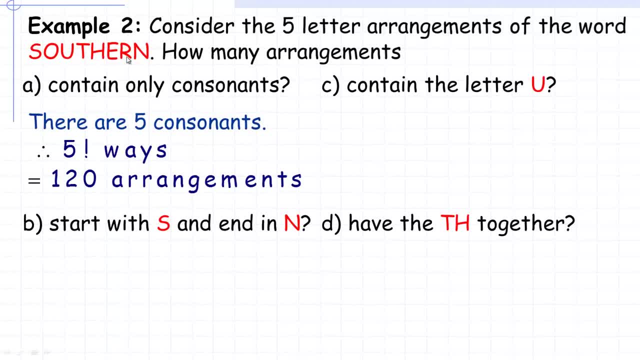 And N with the letter N, So same as in the word southern, Starts with the first letter and ends with the last letter in the word southern. So it would look like this: There's an S at the beginning and there's an N at the end. 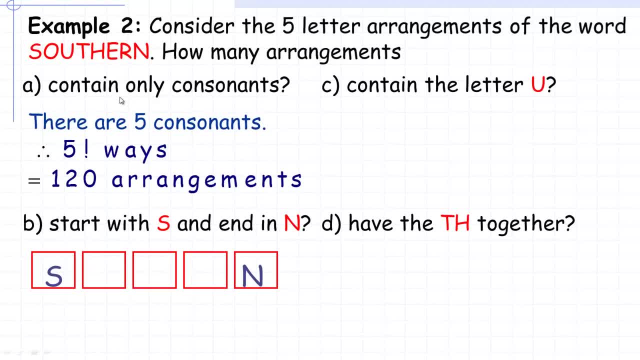 And so in the middle, now, this is independent of A, We're not talking about just consonants, So it can be any. 3 of the other letters from the O, U, T, H, E and R. Now, so there's, if you count them. 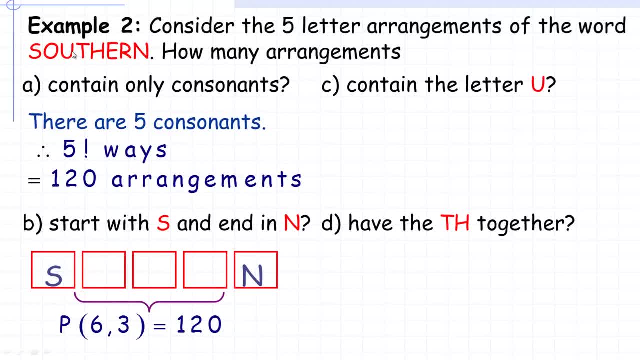 there's 1,, 2,, 3,, 4,, 5, 6 letters between the O and the R, and we're, of course, selecting 3 of them here And we're putting them in different arrangements. That's why this would be a permutation, because, for example, if you go O U T, 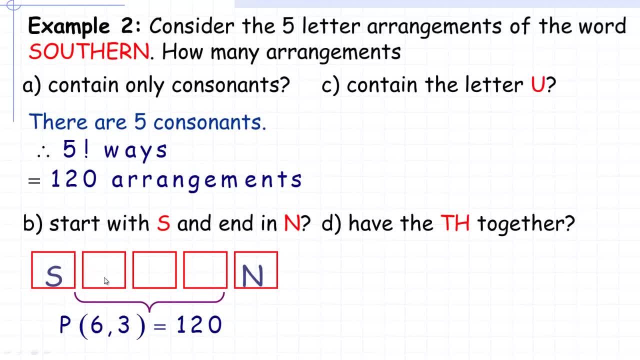 it's different than if you use the same letters but go U T O, for example, in a different order. That's why this is a permutation, So there's only one way to put the first letter, the S, and one letter to put in the end. 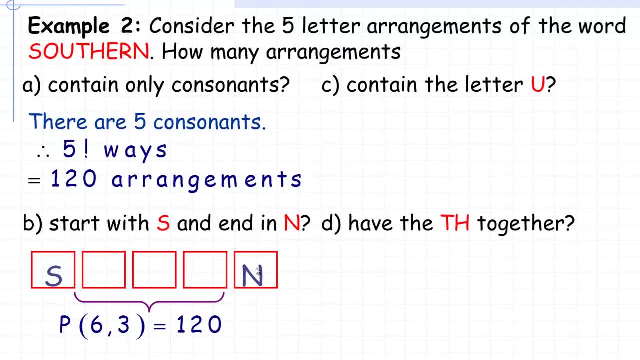 Okay, So they don't have to be in those spots, so they don't change the total number of permutations. The total number of permutations really comes from what's in the middle. that can be in different arrangements, And so that would be 6 permute 3, which is 120.. 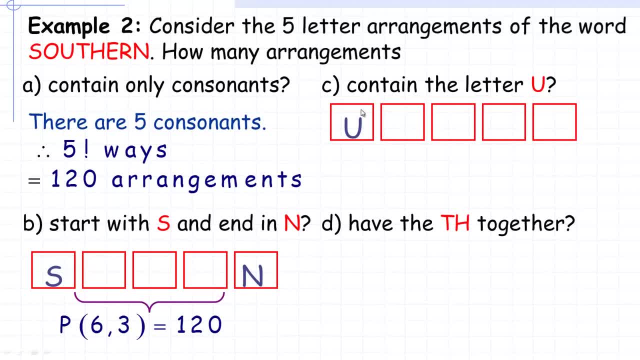 And C says how many contain the letter U. Well, now the U does not have to be just at the beginning, but here there's 5 arrangements here. So let's say the U is at the beginning. The other 4 letters are being selected from the 7 possible letters. 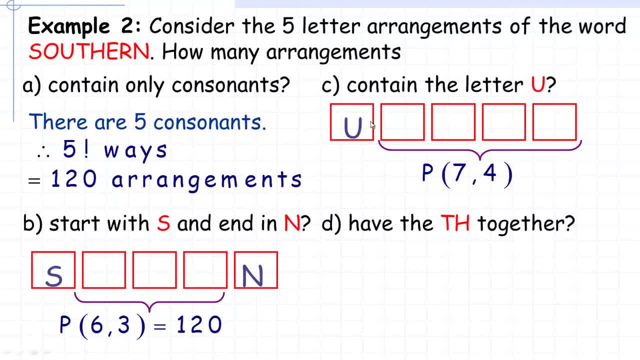 Remember, there's 8 letters here. all together That's the word Southern And we're saying that the? U has to be one of them. So let's say the U is at the beginning. We could arrange these in 7, permute 4 ways. because of the fact that there's 7 objects and we're arranging 4 at a time, we're selecting 4 at a time. 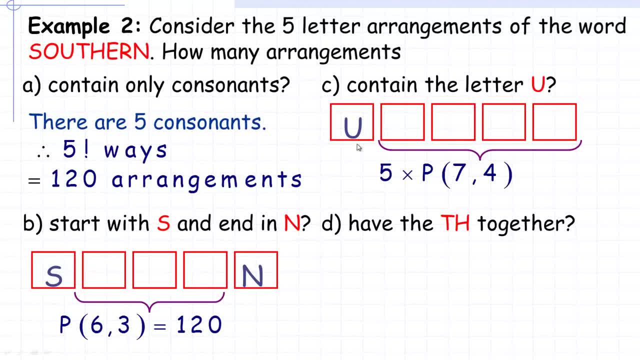 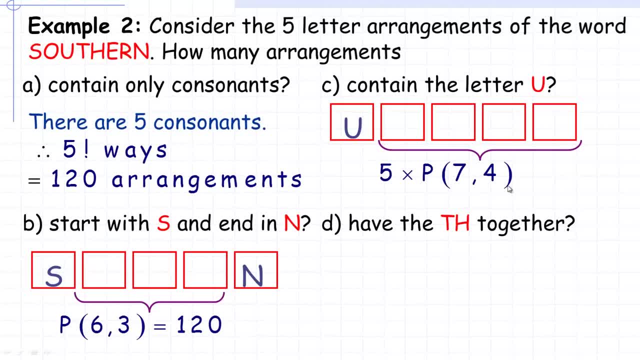 The one that has the U in the second spot there's 7 permute, 4 ways of doing that, etc. So we would multiply by 5, because there's 5 different places the U could be And if we evaluate that, that works out to 4,200.. 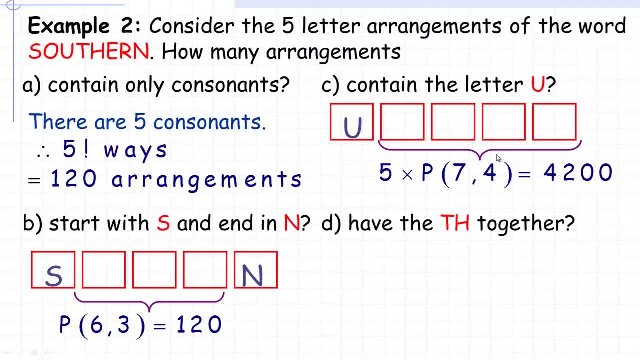 So there's 4,200 ways of selecting 5 letters that have to have the letter U in them For D. how many have the T and the H together? So now there's still 5 letters. So we're saying the T and the H are together. 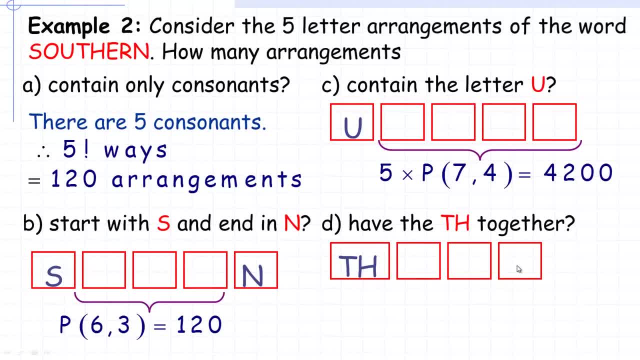 So this is actually 2 places here: T and the H and 3 other letters. And the T and the H do not have to be at the beginning And we'll take care of that, like the U didn't have to be at the beginning here. 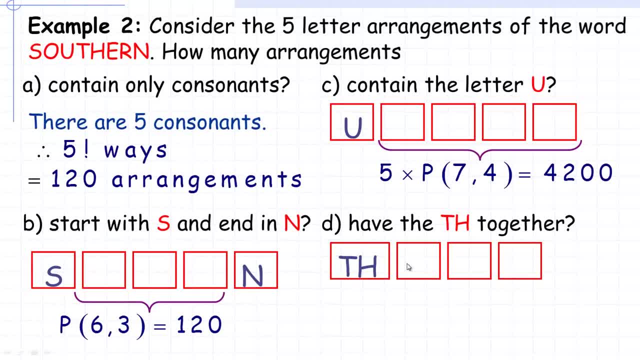 So let's say the T and the H are the first 2 letters. Then, if you remember, there's 8 letters all together. There's 3, 6 other ones if you count them. So there's 6 different letters to go in these spots. 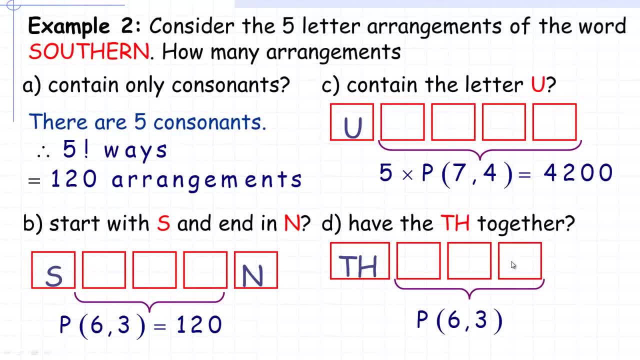 So we could select those in 6 permute 3 ways. We could arrange those in 6 permute 3 ways. So if we're saying the T and the H have to be at the beginning in that order there's 6 permute 3 ways of that particular 5 letter arrangement. 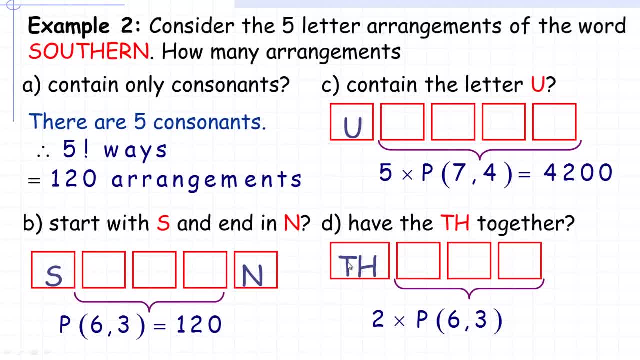 Now, the T and the H could be either T first and H second, or it could be H first and T after it. So that's why we would multiply this by 2, because if there's 2 letters here, there's 2 ways for them to be written. 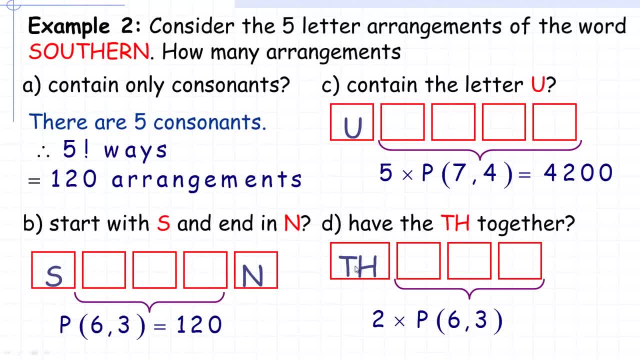 Either the T first or the H first. Now the T and the H could be in the first 2 spots, or the second and third spot, or the third and fourth spot, or the fourth and fifth spot. So there's 4 different ways to do that. 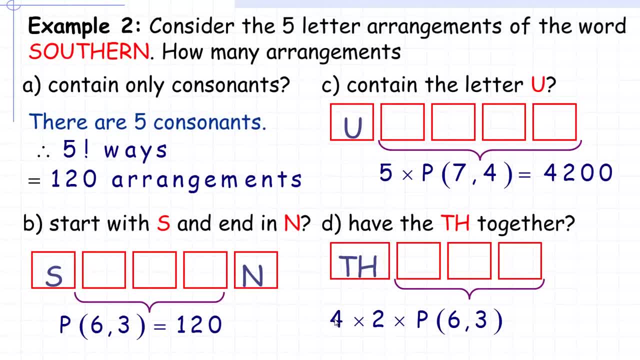 So again, first and second, second and third, third and fourth, fourth and fifth, There's 4 different ways for the places for the T and the H to be, So that's why we would also multiply this by 4.. Kind of like the U could be in 5 different places. 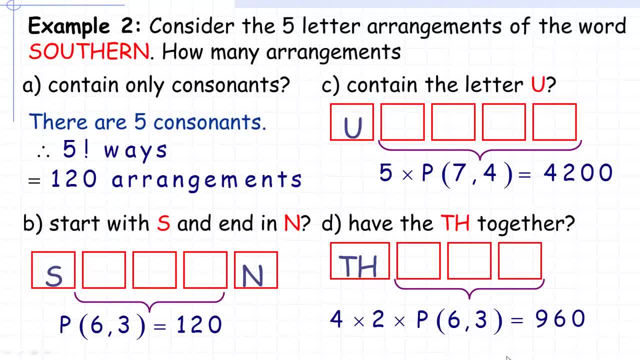 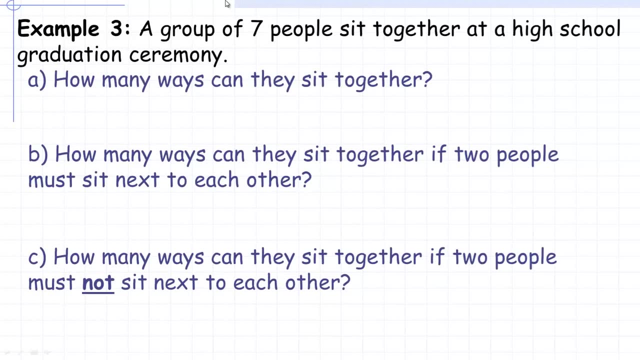 so we multiply it by 5.. So that's the calculation. So a little under 1,000.. There's 960 ways for the T and the H to be together. And example number 3, we've got a group of 7 people that are sitting together at a high school graduation ceremony. 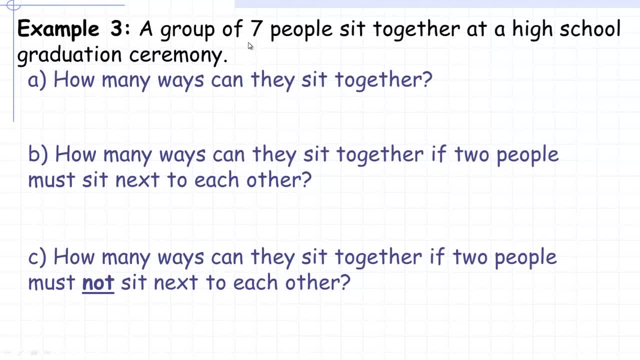 And the first question is: just how many ways can they sit together? So it's an arrangement of 7 people taking 7 at a time. So it's actually the permutation 7, permute 7, which of course would be 7 factorial. 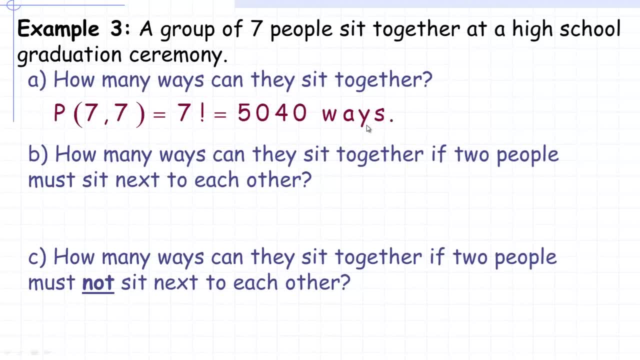 So there's 5,040 ways that they can be arranged. In B it says how many ways can they sit together if 2 people must sit next to each other. perhaps they're a couple or they just want to sit next to each other. 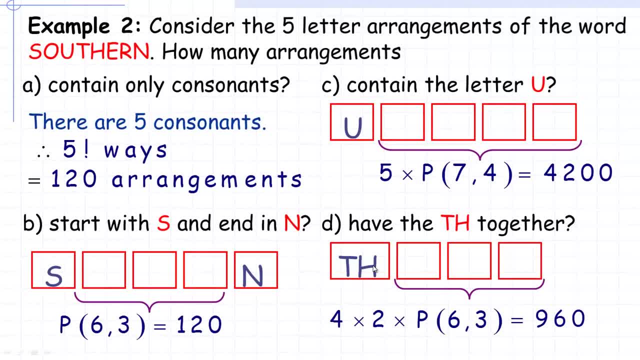 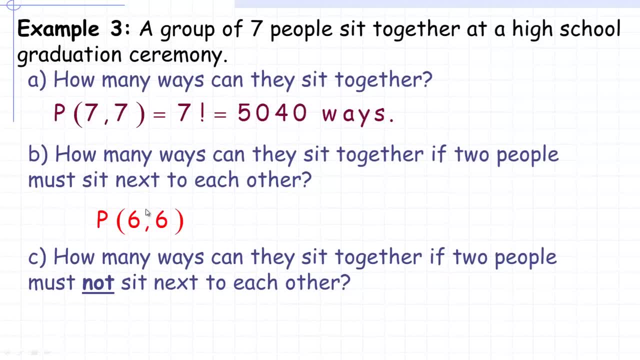 So it's very much like on the previous page: the T and the H, We're putting them together. So if they're together, then think of that as a couple. so that's one object, but it's actually 2 people. 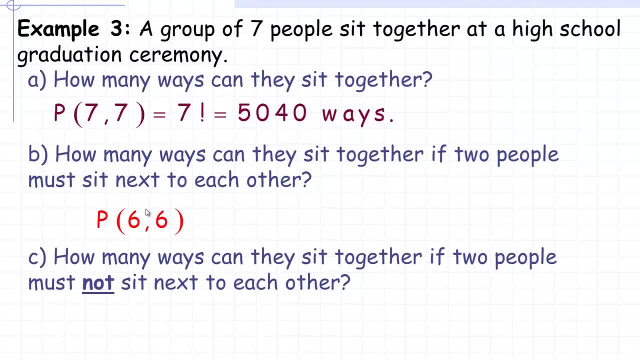 And then there's 5 other people. So there's this pair and there's 5 other people, which makes the 7 all together. So it's really like arranging 6 objects. So we could arrange them in 6, permute 6 ways. 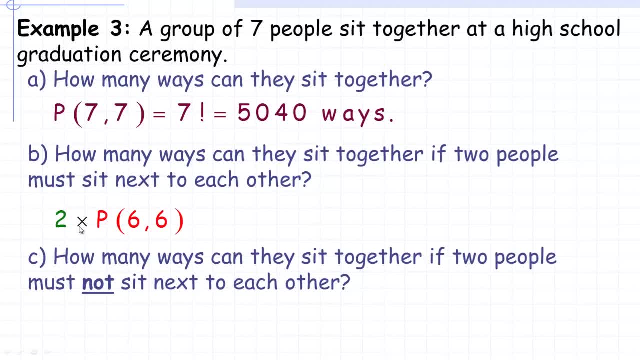 But, like the example on the previous page, we would also multiply that by 2, because let's say it was Henry and Sue. Henry could be first and Sue second, or we could reverse it and put Sue first and Henry second. So that's why we multiply it by 2.. 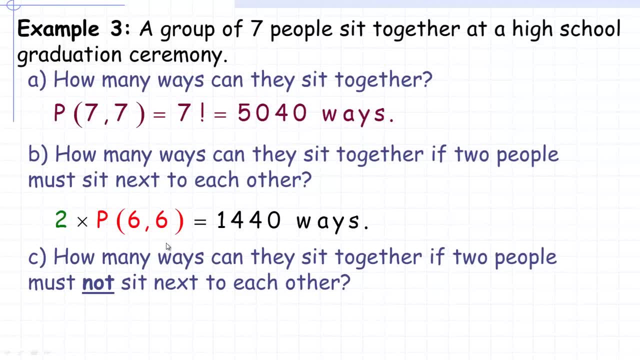 And we don't have to worry about the first and second, second and third, because if they're a couple we're actually saying it can be arranged in the 6 permute. 6 takes care of that, So that works out to 1440 ways. 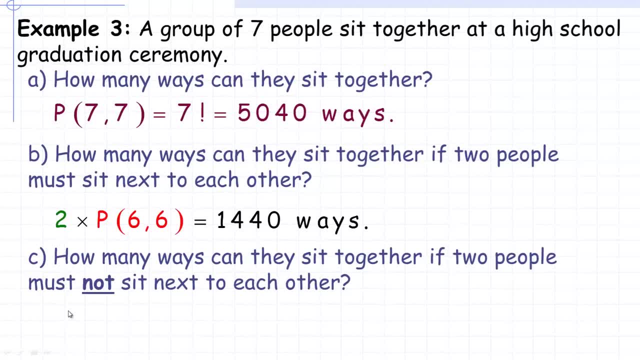 And the last example says: how many ways can they sit together if 2 people must not sit next to each other? So perhaps they're, maybe they're a couple and they had an argument: They don't want to sit next to one another. 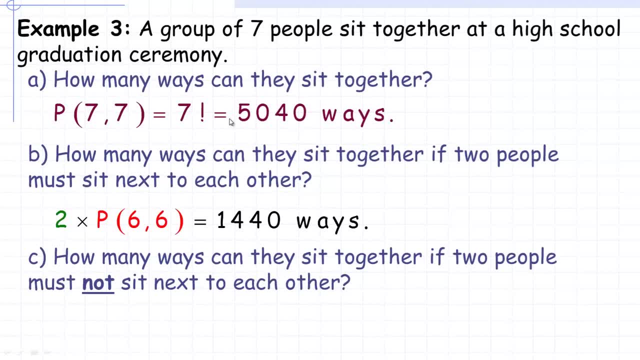 Well, if you think of: OK, this is the total number of ways, that actually OK, there's a long way to do. C You could do. well, perhaps let's say it's Henry and Sue, again, Henry's first and Sue could be third. 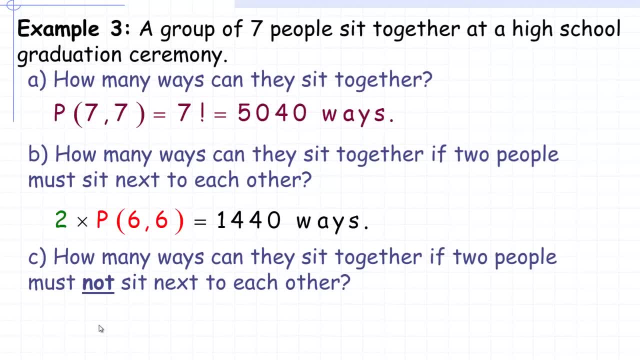 so there's somebody between them in the second spot And Henry could be first and Sue could be fourth. Henry could be first, Sue could be fifth. We could actually calculate all those and add them up And that would be very, very long. 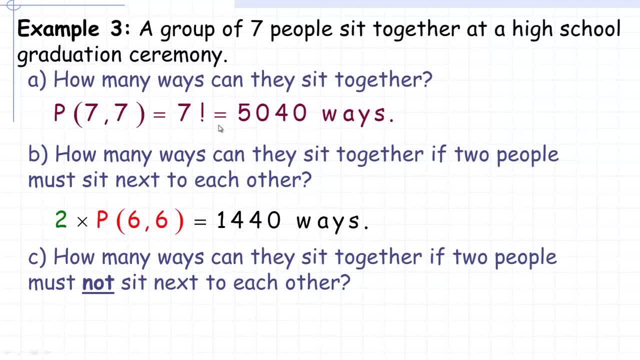 OK, but there is a shorter way to do this. The 5040 is the number of ways that they can be arranged with no restrictions whatsoever. This is the number of ways they can be sitting. they have to be sitting next to one another. 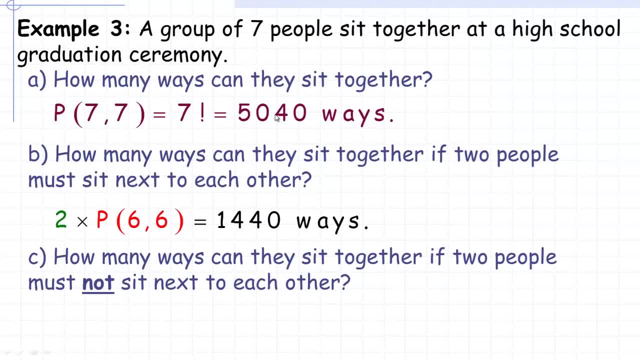 So these two events, this is the total number and this is the number of ways they can sit together This down. what we're looking for down here is an event that's mutually exclusive with this one. They're either sitting next to one another. 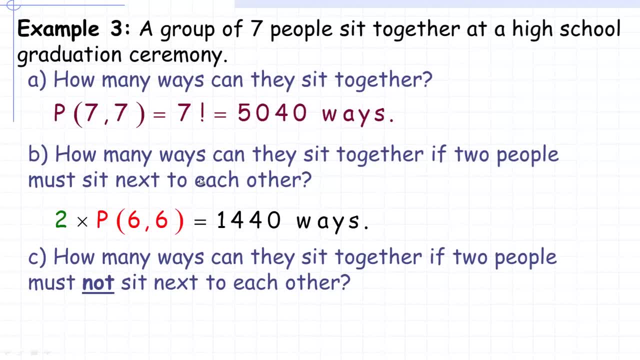 or they're not sitting next to one another. These two answers from B and C should add to the 5040.. Because either they're sitting next to one another or they're not. There's no other possibility. So a quick way to get C is to take the total amount. 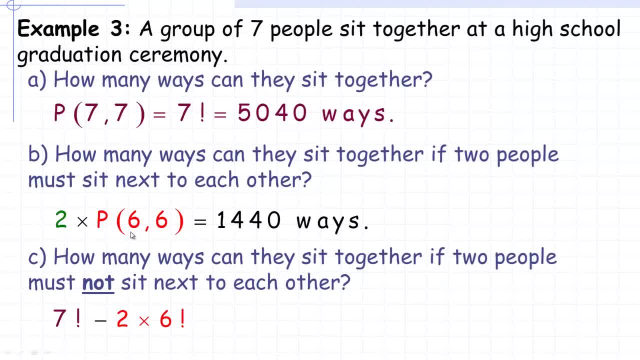 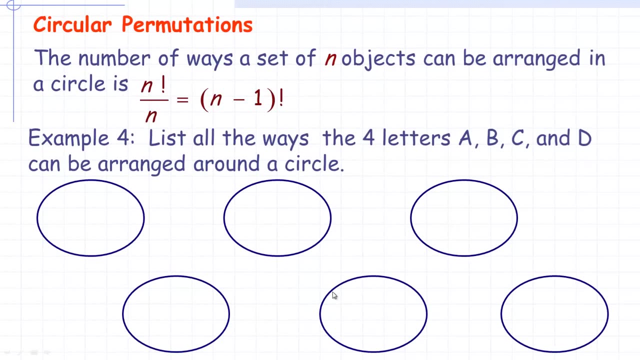 and the 7 factorial and subtract the 1440 from it. So 5040 minus 1440 is 3600 ways. So there's 33,600 ways that they could not sit next to one another. Circular permutations Now. circular just means there's no real start. 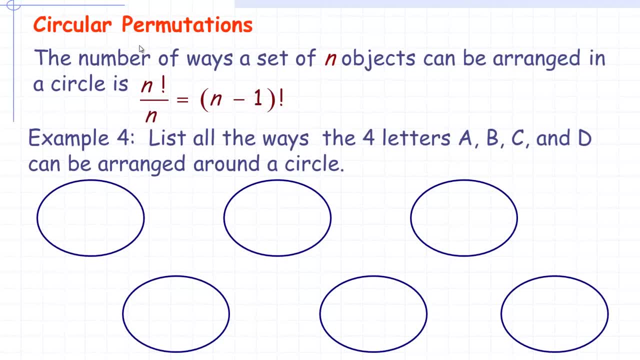 It doesn't have to be around a circle, It could be around a rectangular table, And if there's no start, they're just sitting around it. then that's still referred to as a circular permutation: The number of ways. and when there's no beginning and end. 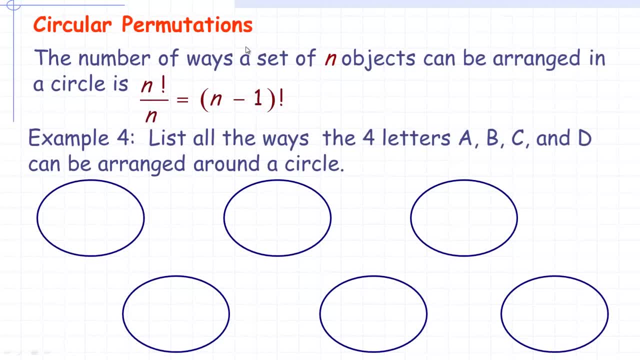 it reduces the number of ways things can be arranged. The number of ways a set of n objects can be arranged in a circle or around something with no start and end is n factorial, N factorial divided by n And n factorial divided by n is actually 1 less than n factorial. 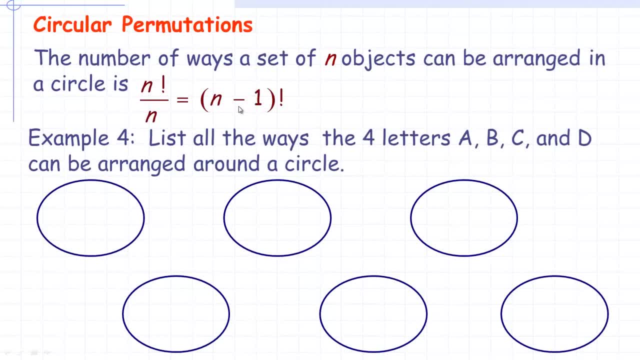 For example, if n was 10, 10 factorial divided by 10 is actually 9 factorial, So it's the number of objects minus 1 factorial. Just to give you an example that that actually works. an example for us is list all the ways: 4 letters. 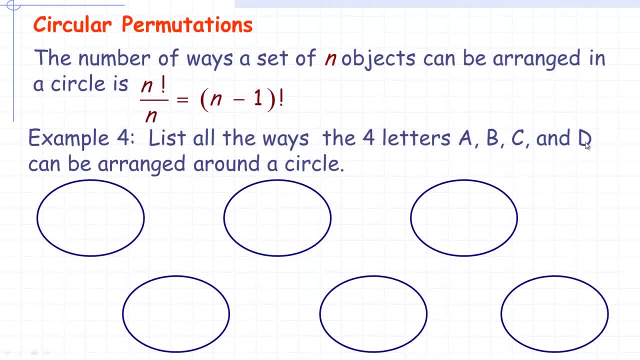 a, b, c and d can be arranged around a circle. Now there's 4 letters. if we use this formula, 4 minus 1 is 3, and so it should be. there should be 3 factorial ways, which is 6.. 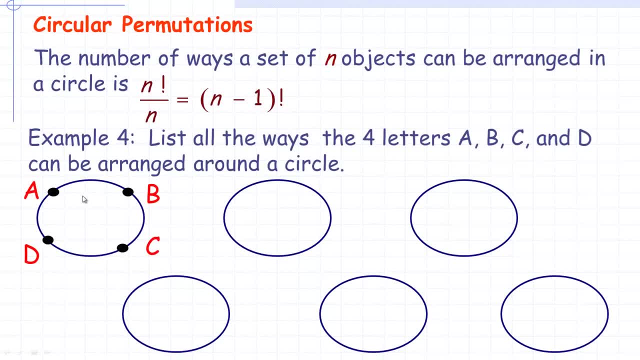 And so if you actually write them all out, so let's say we did a, b, c and d Now, so that's an arrangement around the circle: a first, b second, c afterwards and d afterwards. Now, if I were to put the d up here, 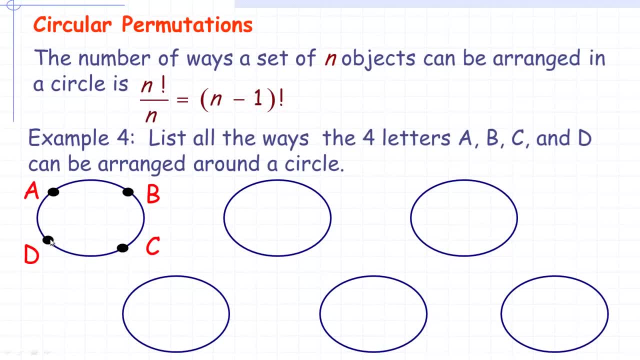 and move the a over here and the b down here and then the c over there. that's the same arrangement. That does not make a different permutation, because it's a certain order around the table, Even if I, you know, move a, two spots. 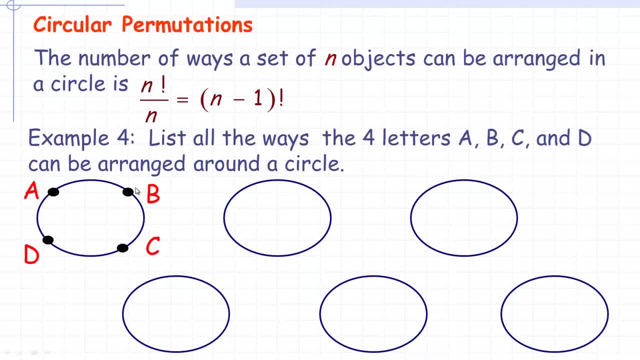 and b, two spots to here and c here and d over here. that's still the same arrangement, because if you go around the circle, let's say clockwise, b is after a and c is after b and d is after c, etc. 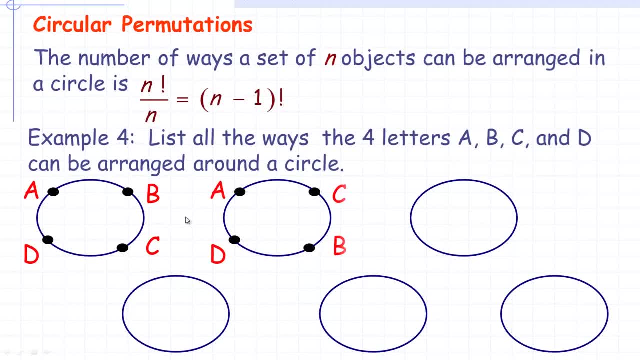 Okay, so that's one way to do it. So, in fact, actually all I'm doing is actually just listing all the different ways, And you could try to, you know, list different ways around the circle, but those are actually all of them. 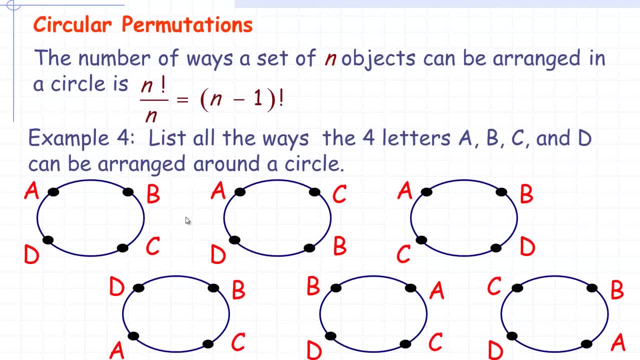 Those are all the different orders, that you could put four things around a circle or a rectangle or whatever. So that actually just is a demonstration that this formula works. It's not a proof, It's just an example with four objects. 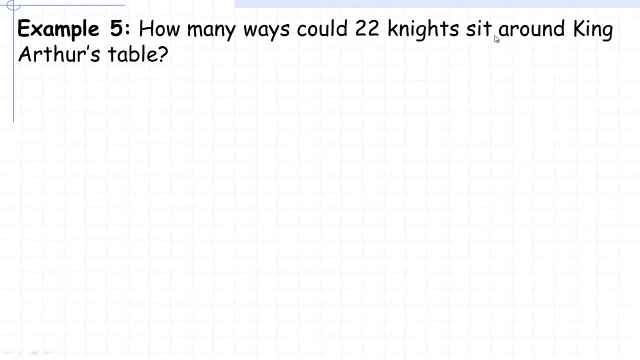 One last example: How many ways could 22 knights sit around King Arthur's table? So here's a circular permutation: They're sitting around. remember his table actually was supposed to be round. So it's 22 objects. So we would evaluate 21 factorial.